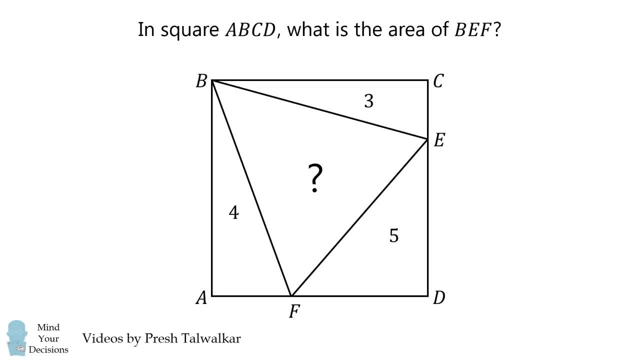 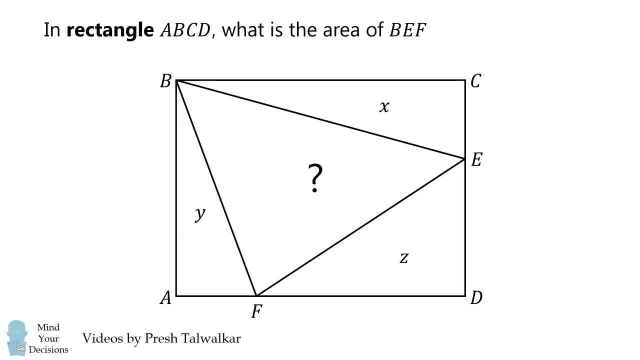 of Mathematics. For a little bit more of a challenge, consider the general case where ABCD is a rectangle and the areas are X, Y and Z. What is the area of BEF in terms of X, Y and Z? This comes from a tweet by Mustafa Kemal Inca. Pause the video if you'd like to give this. 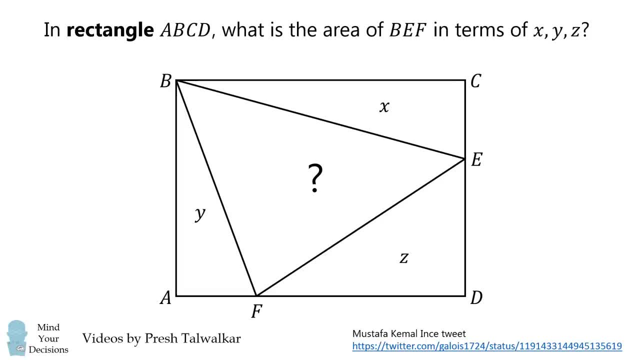 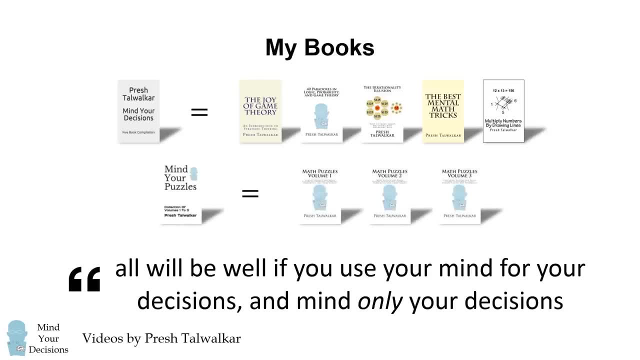 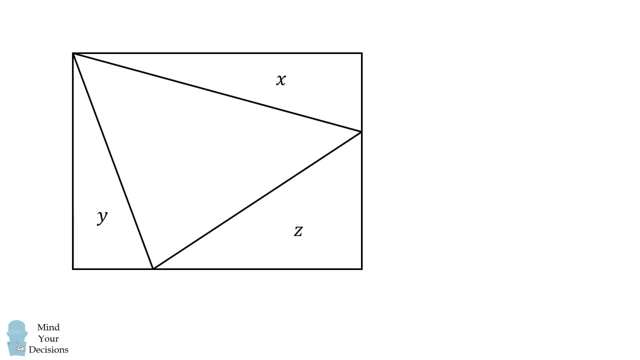 problem a try and, when you're ready, keep watching to learn how to solve this problem, The General Case. We'll go ahead and tackle the general case and we'll prove the following formula To do that. we'll work step by step. 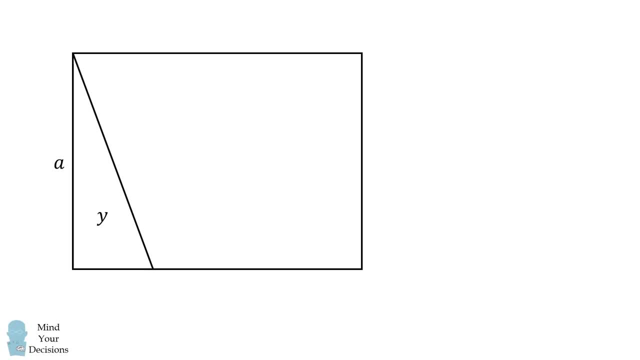 First consider this triangle. Suppose one side of the rectangle is A and the other side of the triangle is C. Because the triangle has an area of Y, AC over 2 is equal to Y. This means C is equal to 2Y over A. Now suppose the other side of the rectangle is B. 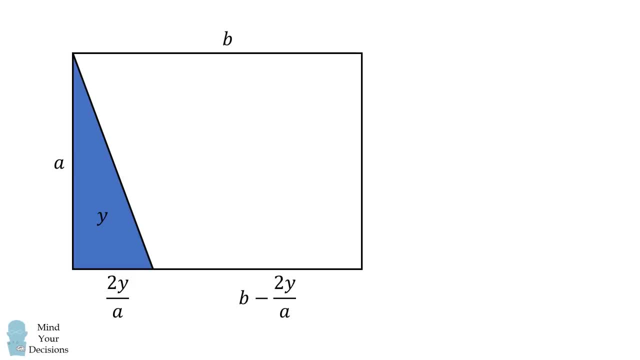 The remaining distance on this side will be b minus 2y over a. Now consider the triangle which has an area of x. If its other side is equal to d, we can solve that bd over 2 is equal to x. This means d is equal to 2x over b. 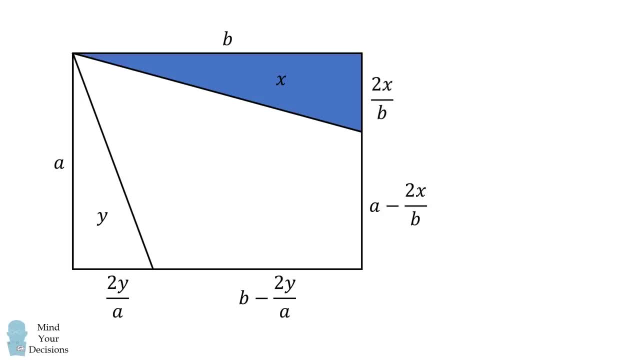 The other distance on this side will be a minus 2x over b. We have the final triangle with an area of z, So we can set that 1 half times each of its legs will be equal to the area of z. We'll then focus on this equation. 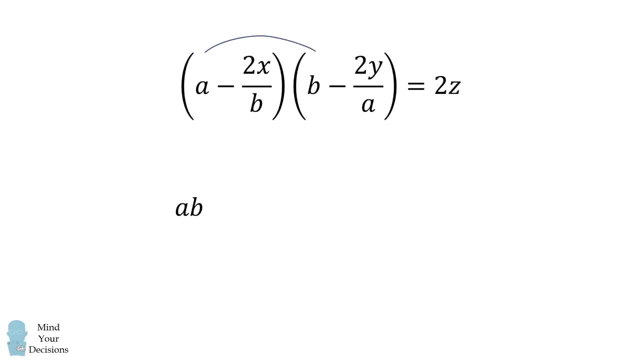 First we'll multiply both sides by 2, and then we'll distribute this binomial. Now it looks pretty complicated, but it's going to simplify. The first thing we'll do is we'll subtract 2z from both sides. We'll then factor a 2 from these three terms. 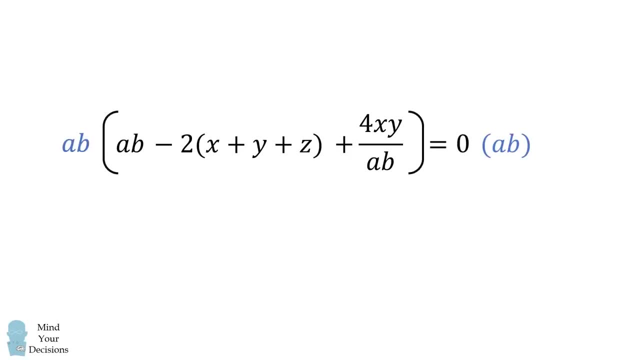 Now let's multiply. We'll multiply both sides by the quantity ab. On the right hand side, this will vanish, because 0 times ab is equal to 0.. On the left hand side, we'll distribute it over three different terms. The first term becomes ab, the quantity squared. 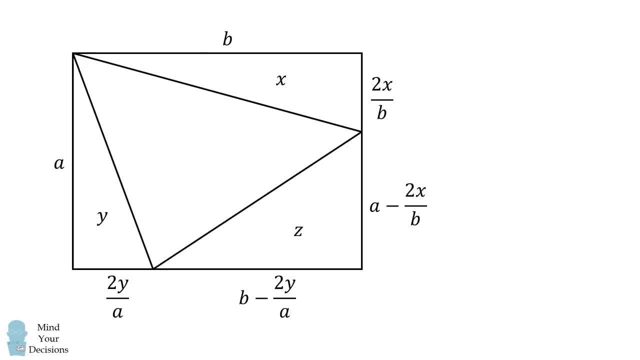 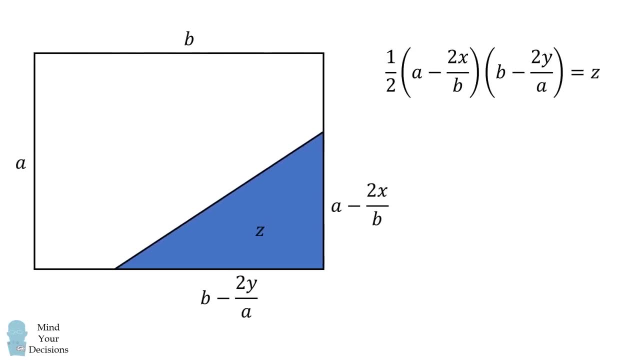 We have the final triangle with an area of z, So we can set that 1 half times each of its legs will be equal to the area of z. We'll then focus on this equation. First we'll multiply both sides by 2, and then we'll distribute this binomial. 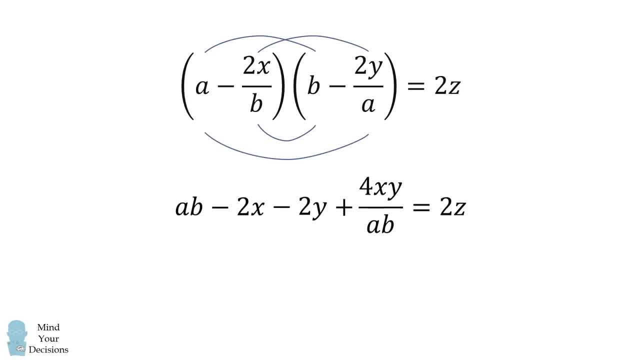 Now it looks pretty complicated, but it's going to simplify. The first thing we'll do is we'll subtract 2z from both sides. We'll then factor a 2 from these three terms. Now let's multiply. We'll multiply both sides by the quantity ab. 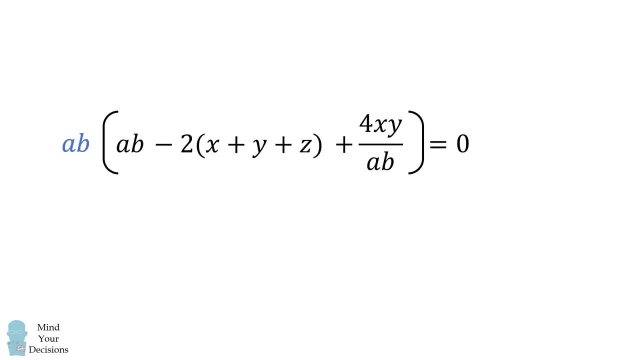 On the right hand side, this will vanish because 0 times ab is equal to 0.. On the left hand side, we'll distribute it over three different terms. The first term becomes ab, the quantity squared. The second term: we add a factor of ab. 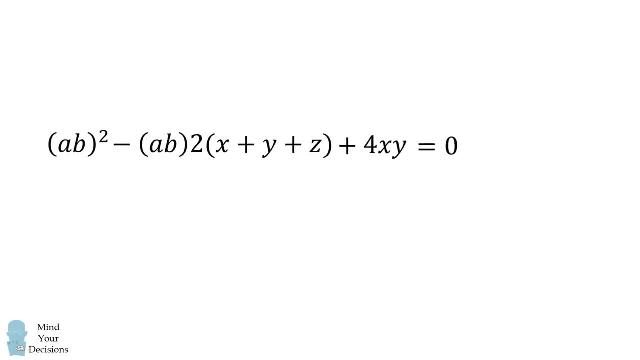 And the third term, the denominator of ab, will vanish. This equation looks complicated, but it's actually something you should be able to solve. This is going to be a quadratic equation in the variable ab, So we can use the quadratic formula to solve it. 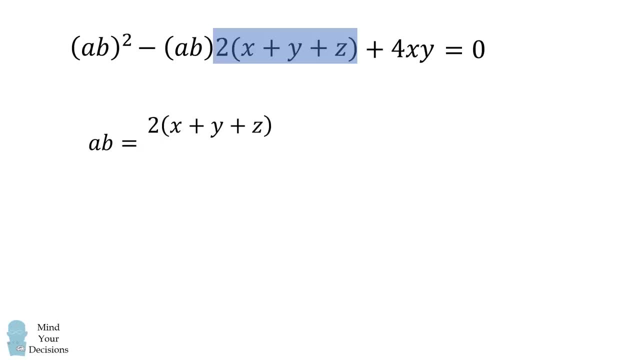 ab will be equal to the opposite of the coefficient on ab plus or minus, the following: all over 2.. We then will simplify the square root by factoring out a, 2, and then these factors of 2 will all cancel out. So ab will be equal to x plus y plus z plus or minus. 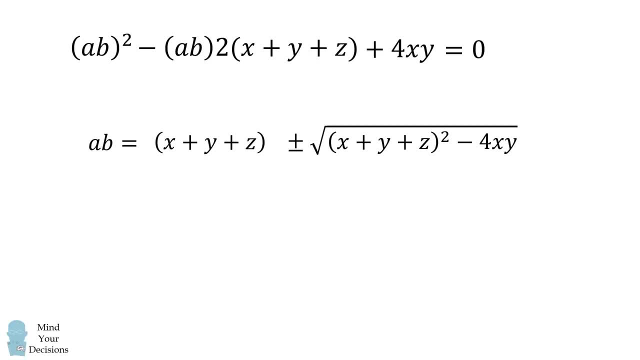 the following square root. Now it looks like we have two choices plus or minus, but here's how we can rule out one of the choices. Recall that ab is equal to the area of the rectangle and that has to be larger than x plus y plus z. 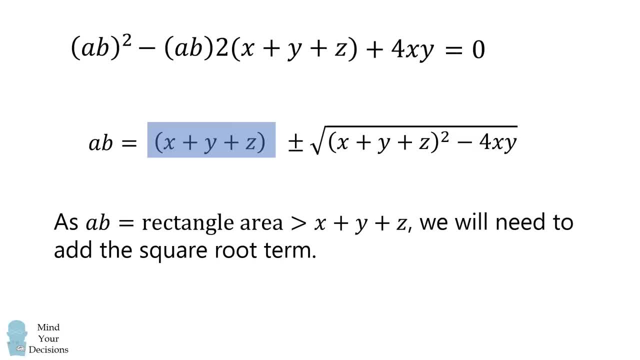 because those are the areas of those three triangles. Since ab is larger than x plus y plus z, we will need the positive square root. We don't want to subtract anything from it. The area is going to be larger than the areas of the three triangles. 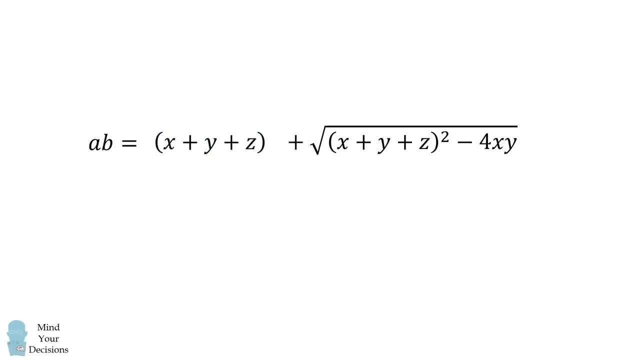 So we eliminate the negative term and we have an answer for what ab is equal to. Now go back to the original diagram. The entire area of the rectangle is ab, So ab will be equal to the entire area, but it's also going to be equal to the sum of the areas of these triangles. 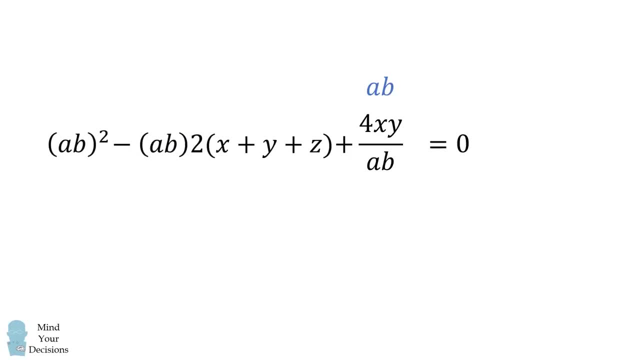 The second term, we add a factor of ab And the third term, the denominator of ab will vanish. This equation looks complicated, but it's actually something you should be able to solve. This is going to be a quadratic equation in the variable ab. 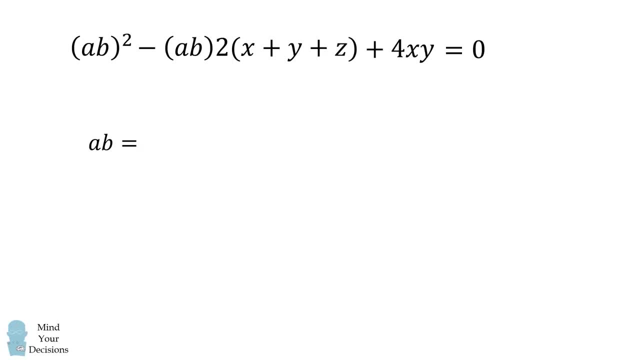 So we can use the quadratic formula to solve it. ab will be equal to the opposite of the coefficient on ab, plus or minus the following: all over 2.. We then will simplify the square root by factoring out a, 2, and then these factors of 2 will all cancel out. 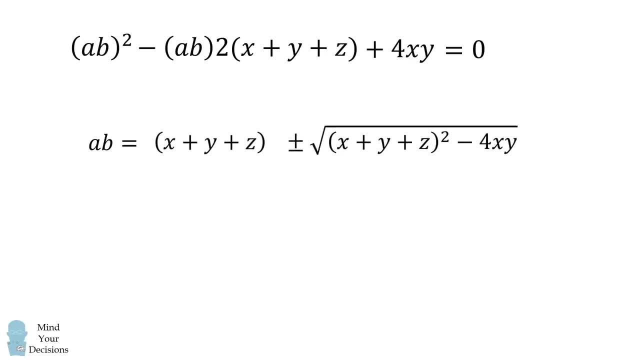 So ab will be equal to x plus y plus z, plus or minus the following square root. Now it looks like we have two choices, plus or minus. but here's how we can rule out one of the choices. Recall that ab is equal to the area of the rectangle and that has to be larger than x plus y plus z. 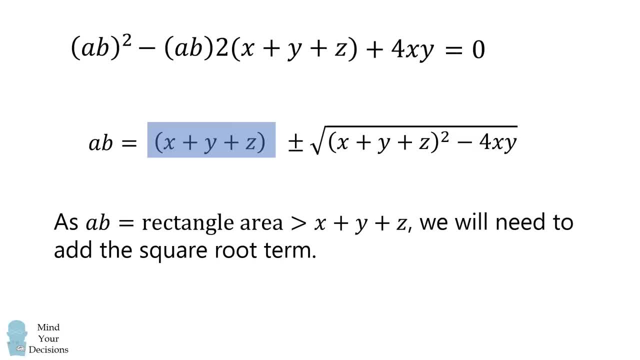 because those are the areas of those three triangles. Since ab is larger than x plus y plus z, we will need the positive square root. We don't want to subtract anything from it. The area is going to be larger than the areas of the three triangles. 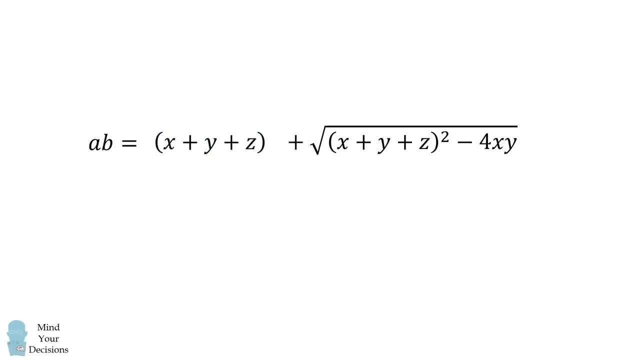 So we eliminate the negative term and we have an answer for what ab is equal to. Now go back to the original diagram. The entire area of the rectangle is ab, So ab will be equal to the entire area, but it's also going to be equal to the sum of the areas of these triangles. 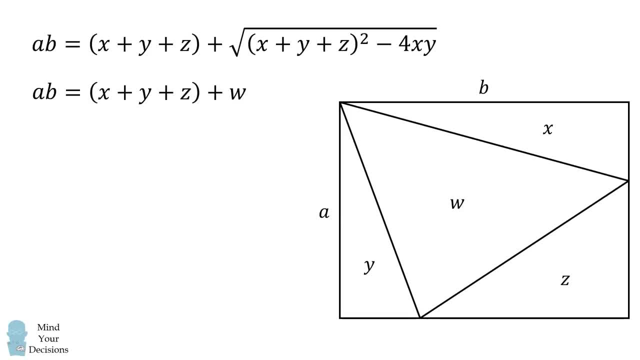 So it's also equal to x plus y plus z plus w. We have two different equations for ab. Therefore we must have the following two terms: This means w is equal to the square root of the quantity x plus y plus z, squared minus 4xy. 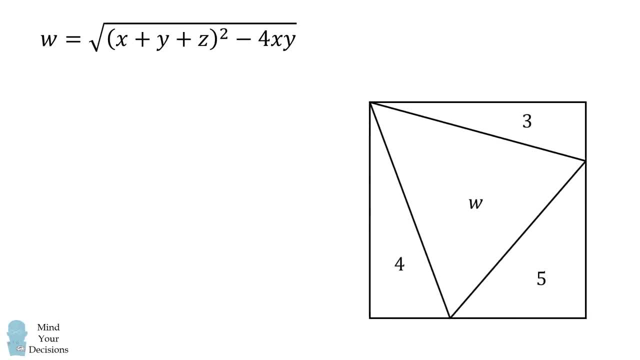 And that's going to be the formula we use. So go back to the original problem, where we have 3,, 4, and 5.. We can easily solve for w by substituting in and then simplifying: w is equal to 4 times the square root of 6,, which is approximately equal to 9.80, and that's our answer. 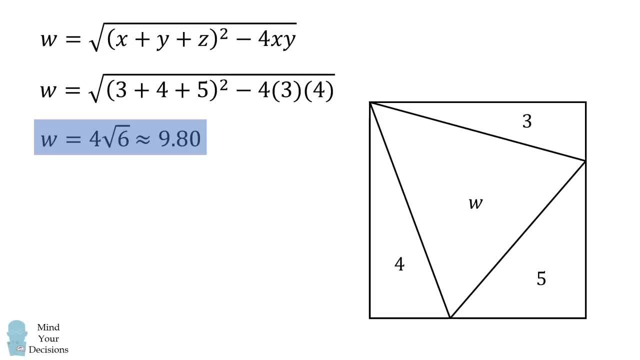 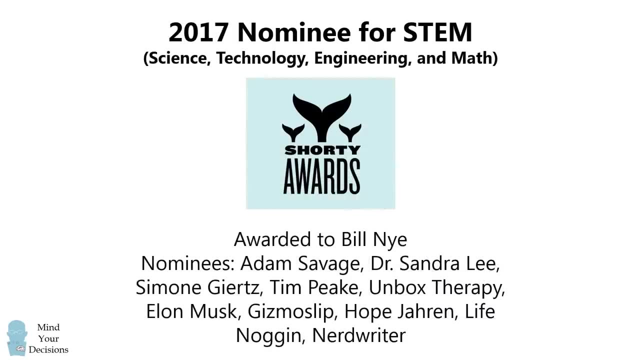 I think it's incredible that there's such a simple formula to solve all problems of this type. Thanks for making Mind Your Decisions. one of the best channels on YouTube. As always, thanks for watching and thanks for your support.